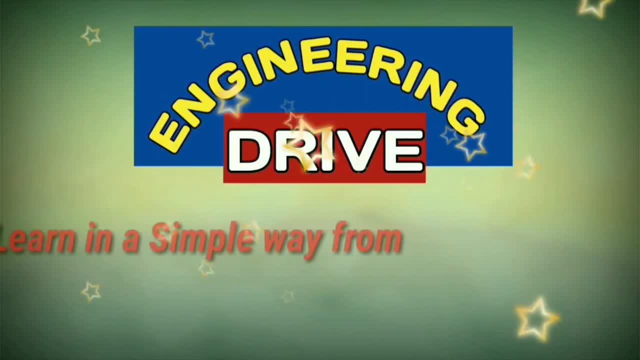 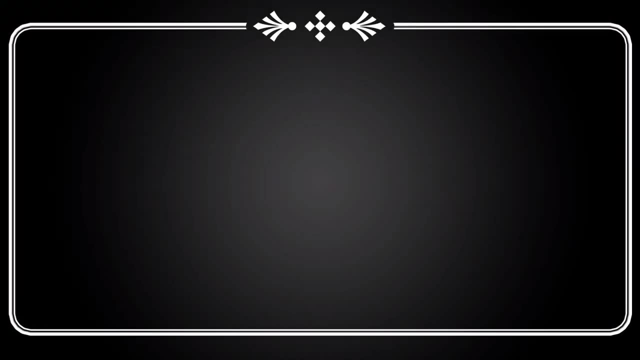 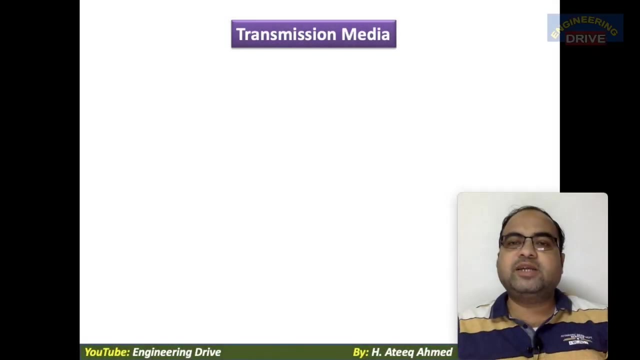 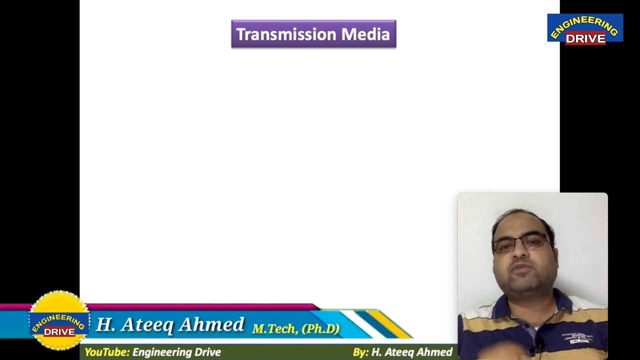 Hi, everybody, hope you are all fine. This is Atiq. Welcome to our YouTube channel, Engineering Drive. Let me discuss the concept of transmission media in computer networks, And I believe that without this topic of transmission media, there will be hardly any type of question paper related. 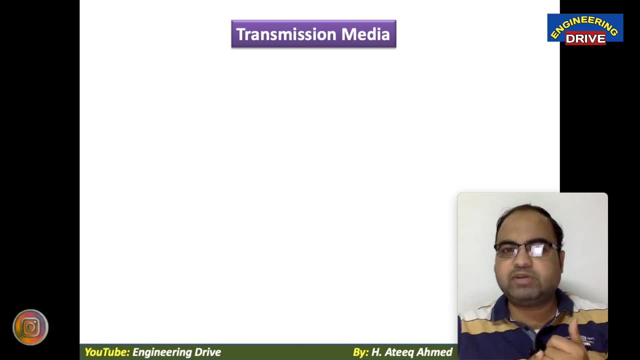 to computer network subject. If you take any competitive exam, or if you take any public examination or any external exam, I believe that there will be no question paper without this transmission media concept. So, dear students, this is very, very important topic of the subject. 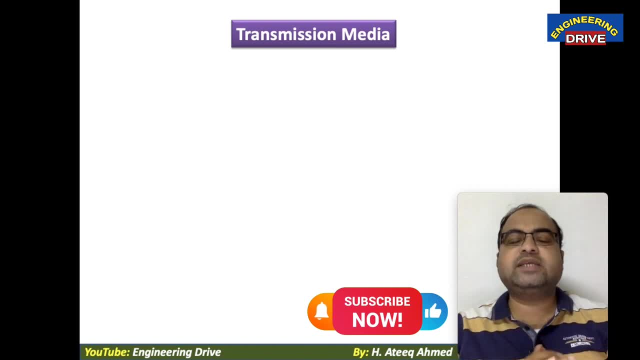 computer networks. Now, without wasting the time, let me start. what is transmission media? A transmission medium can be broadly defined as anything that can carry information from a source to a destination. So, dear students, we know that in computer networks one device want to communicate with another device. how they can communicate with each other? by passing. 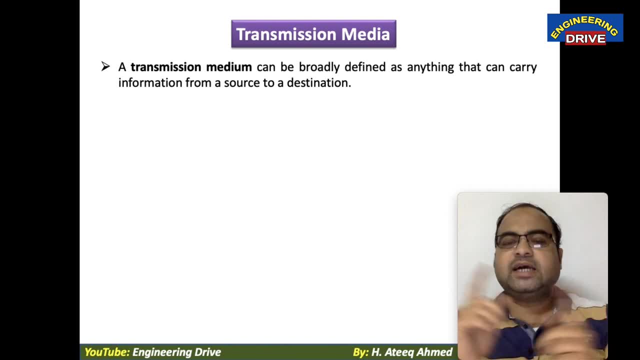 the messages, or by sending the messages, or by sending the information. Now, source can send the information to destination. sender can send the information to receiver with the help of transmission media. Ok, this is what transmission media is all about. Ok, for example, the transmission medium. 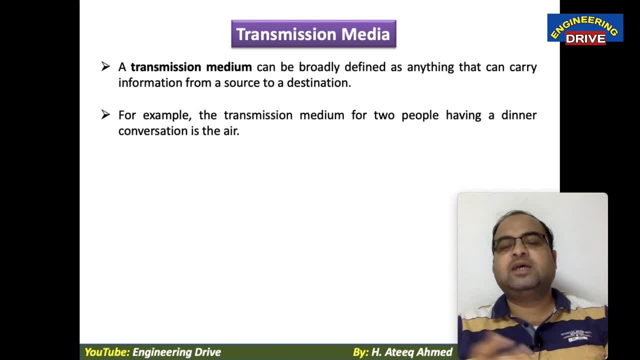 for two people having a dinner conversation is the air. Let us say two people are having a dinner and if they are talking with each other, then what is the transmission between transmission media between them? Of course it is air. Ok, we can't say there is a cable. 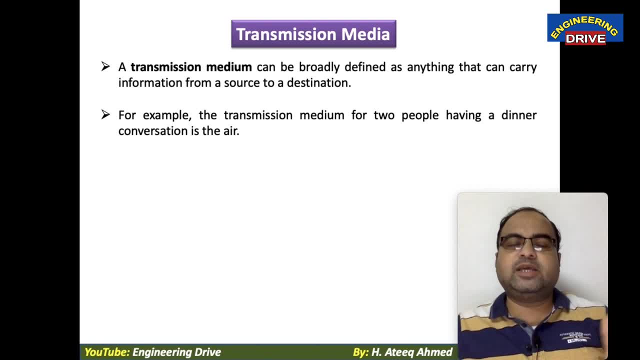 available between them. There is no physical medium available there, available between them. what is the media between their conversation? is air, Ok. next thing: the transmission medium is usually free space- metallic cable or fiber optic cable- So transmission medium can be anything like a free space, like just now I told two people chatting while having a dinner. 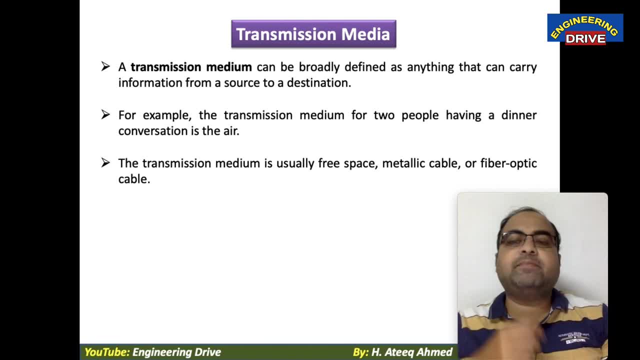 free space, that is, air, or it can be a physical media like a metallic cable or even a fiber optic cable. Ok, So transmission media are actually located below the physical layer and are directly controlled by the physical layer. So where is the location of this transmission media? 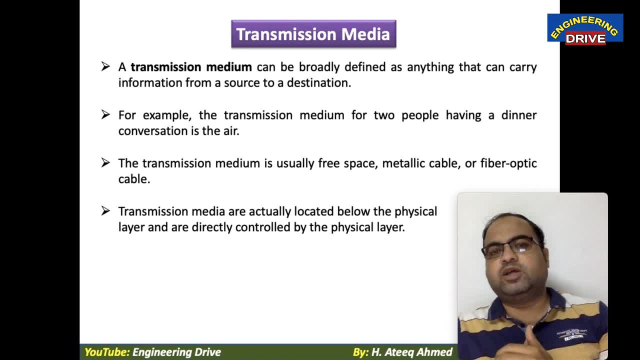 We know that there are seven layers in the OSI reference model. Now, in this, where is the place of this transmission media? It is just below the physical layer. So let me show you the diagram now. You can see here, dear students, this is a sender and receiver, and 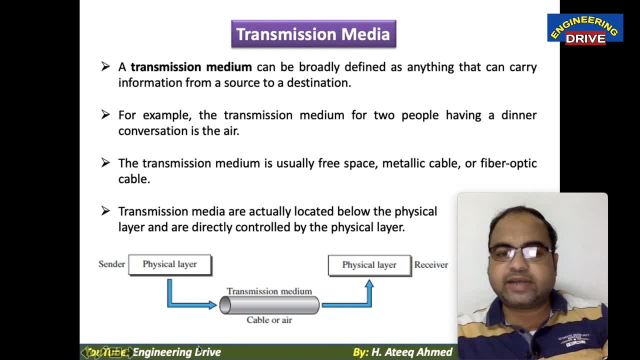 if they want to communicate with each other, then they will make use of some transmission medium, the transmission medium or a channel. now, this transmission medium can be a cable or air. so what is a cable? it is a physical medium, and air is nothing but which is a not a physical medium. 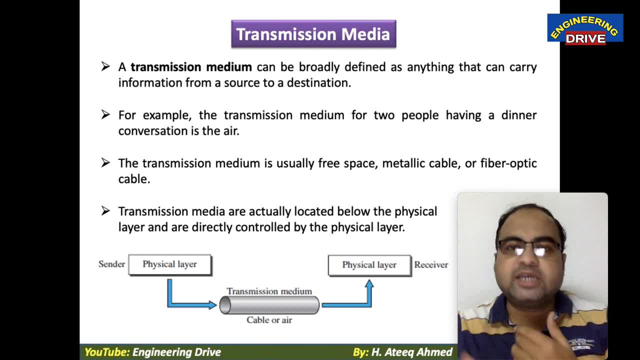 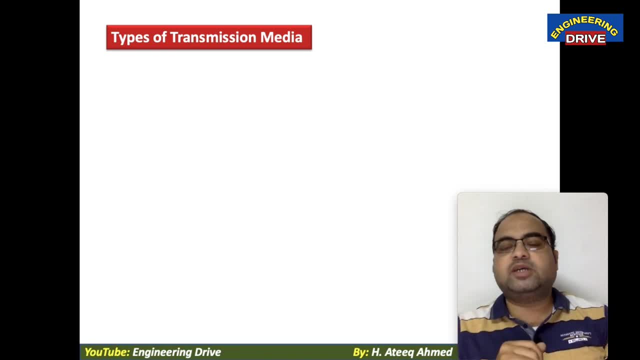 either by using a physical medium or by not using a physical medium, transmission can take place, is it right? types of transmission media. so what are the types of transmission media available and which is supported by computer networks? in telecommunications, transmission media can be divided into two broad categories. one is guided, another one is unguided media. so this 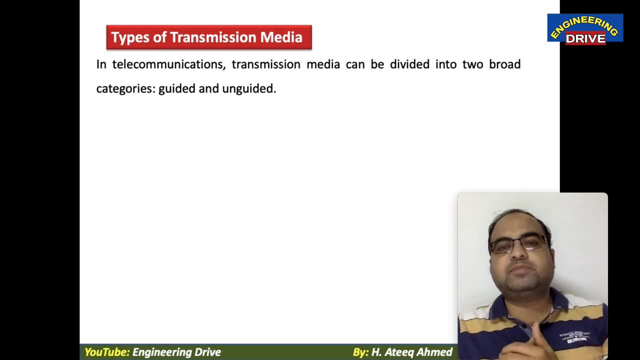 is very, very important question. so what are the types of transmission? media means two categories: guided media and unguided media. okay, if we concentrate on the sighted itself, we will get some idea what is the meaning of guided media and what is the meaning of unguided media. so let me 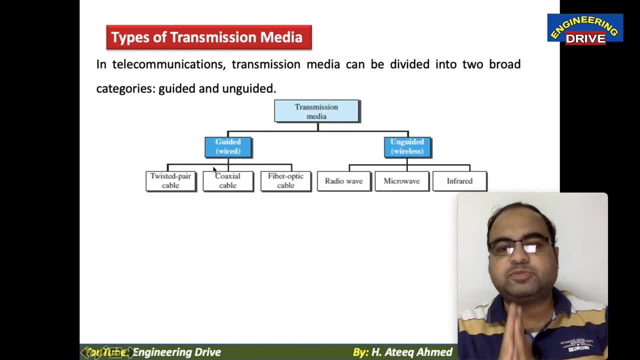 show you this diagram. this shows the classification of this transmission media, is it right? you can see here, transmission media is classified into two categories: guided and unguided. what is the difference between guided media and unguided media? here i have told already: guided media is nothing but wired media, unguided. 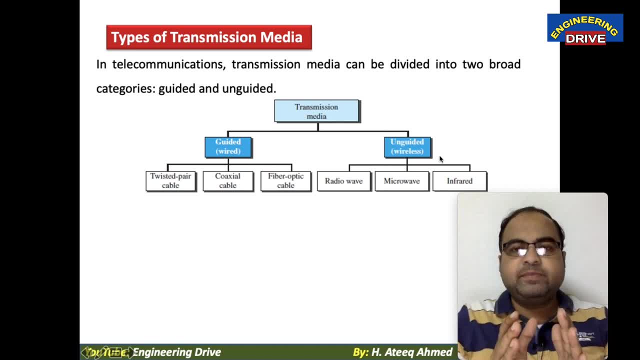 media is nothing but wireless. so which means in guided media there will be some physical connection between or among the devices, whereas coming to the unguided media, there is no physical connection in between the devices or among the devices. so that's why we are calling it as wireless guided. 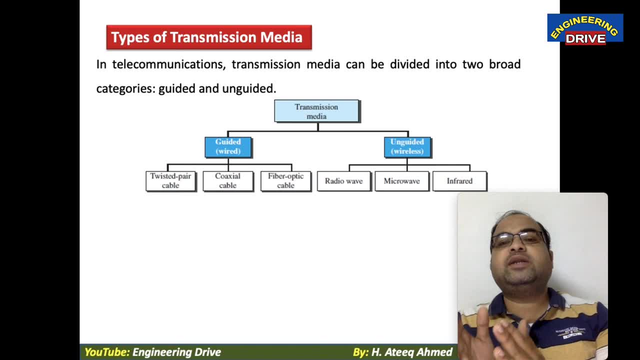 media means in the presence of wire. unguided media means without the help of any wire or physical connectivity. is it ok now? there are three categories in guided media. how many types? three types: twisted pair cable, coaxial cable or fiber optic cable. by using any of these three, we can 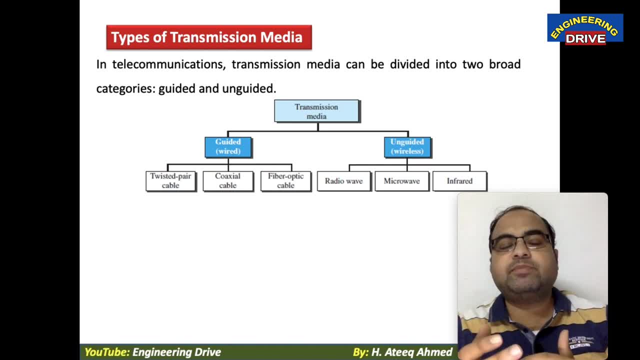 achieve the performance of a wired or unguided media- so this is one of the three categories- In such a way that the data can be transmitted through physical medium. Similarly, while coming to the unguided media or wireless media, We have similarly three categories: Radio waves, microwaves and infrared waves. 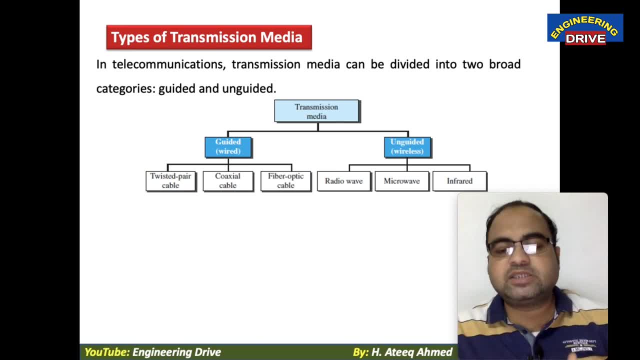 So we will discuss them in detail in our next sessions. Next point: Guided media are those that provide a medium from one device to another. So guided medium is just now I told There will be physical connectivity between the devices From sender to receiver. Guided media include twisted pair cable, coaxial cable and fiber optic cable. 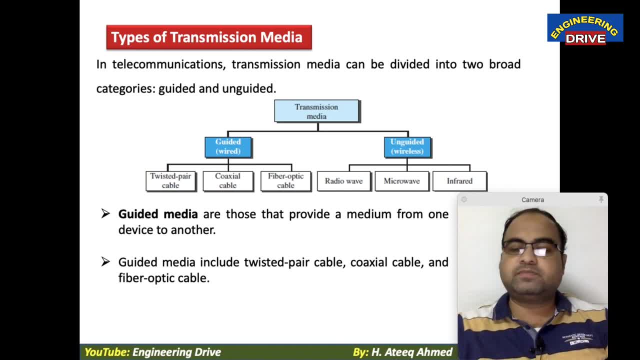 So these are the three examples of guided media, Is it okay? And next, A signal traveling along any of this media is directed and contained by the physical limits of the medium. So, dear students, you can see here, Based on the limit of the physical connectivity, The data will be transmitted from source to destination. 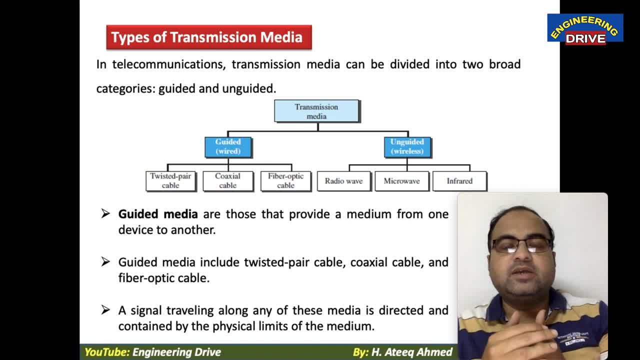 Whereas in unguided media there will be no limit. It depends on the type of wireless media that will be used. Okay, Now You people will have one doubt, Sir: what is the difference between guided media and unguided media, And which is best one, sir? So can you elaborate? 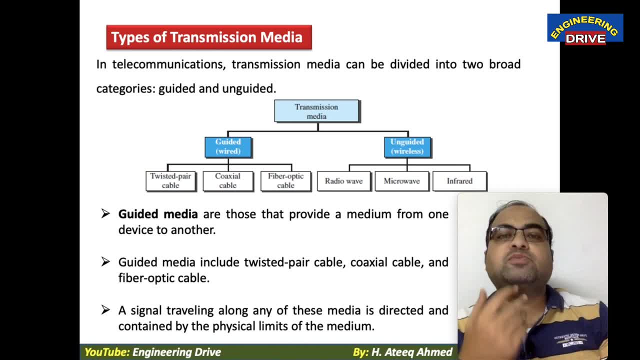 What is twisted pair cable? What is coaxial cable? What is fiber optic cable? Then, what is radio waves, What is microwaves And what is unguided media, And what is infrared waves? So, dear students, In my next sessions of computer networks, I will be discussing in detail about what is guided media. 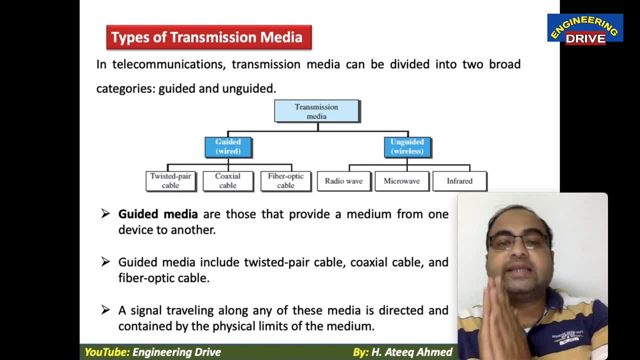 And in my next further session I will be focusing on what is unguided media And what are the types of unguided media in detail. So any types of questions, you can simply put it in the comment section. So with this let me close my today's session of video. 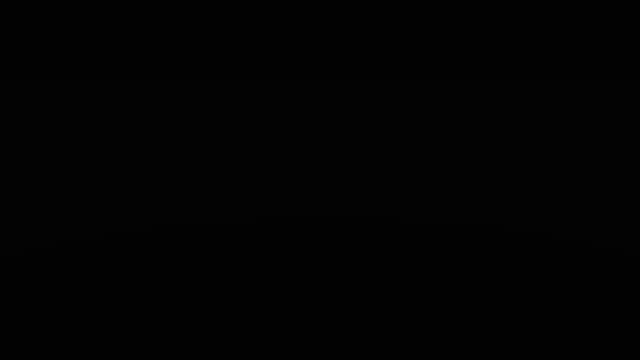 See you soon, everybody, Take care. Allah Hafiz Al Fatiha.